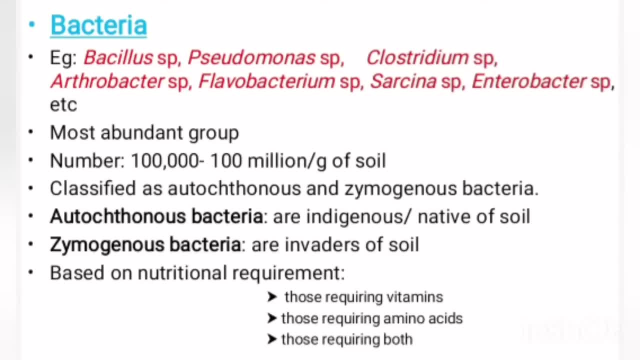 Arthrobacter, Enterobacter Salcina, Flavobacterium, etc. Based on the ecological differentiation, soil bacteria are classified into Autochthonous bacteria and Zymogenous bacteria. Autochthonous bacteria are indigenous or native of the soil and their population. 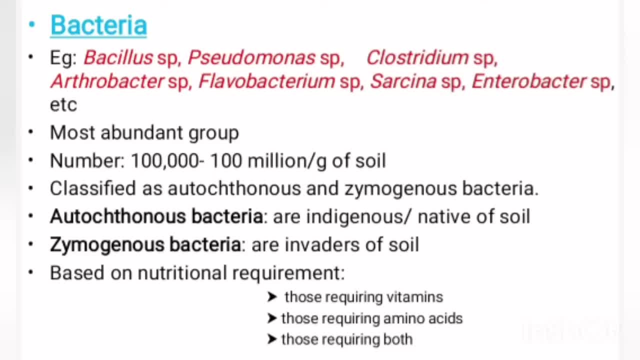 is uniform. Zymogenous bacteria are the invaders of soil and their population depends upon the source of energy. Their normal population is low, but when a specific substrate is added to the soil they increase in number. Based on the nutritional requirement, soil bacteria are classified as those requiring 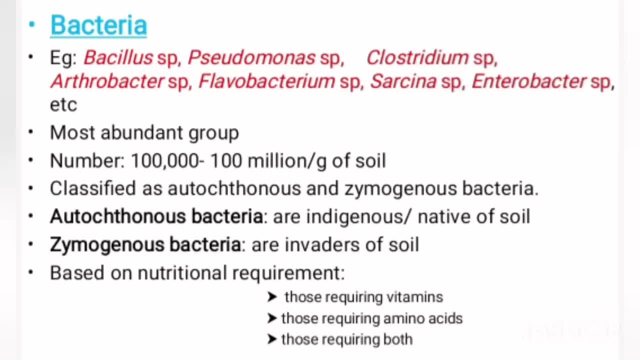 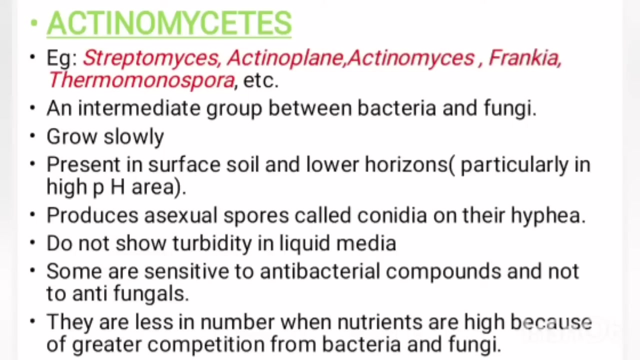 amino acid, those requiring vitamins and those requiring both. Based on the temperature requirement, soil bacteria are classified into mesophiles, thermophiles and psychrophiles. Second group of soil microorganism is actinomycetes. Examples for the actinomycetes: 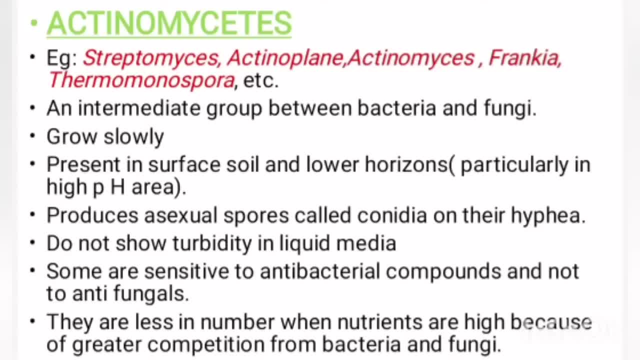 are streptomyces, actinomyces, actinoplane, frangia, thermomonospora, etc. Actinomycetes are intermediate group between bacteria and fungi. They are less in number when the nutrient is high. because greater competition from bacteria and fungi Actinomycetes are. 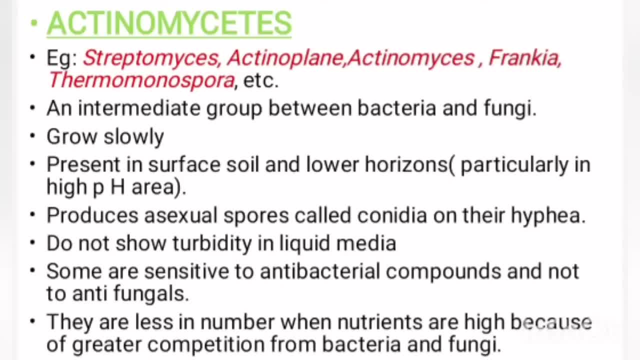 sensitive to the antibacterial compounds and not to antifungal compounds. Actinomycetes grow very slowly and they do not show turbidity when grown in liquid culture. It produces asexual spores called conedia, on their hyphae Taxonom tenho. 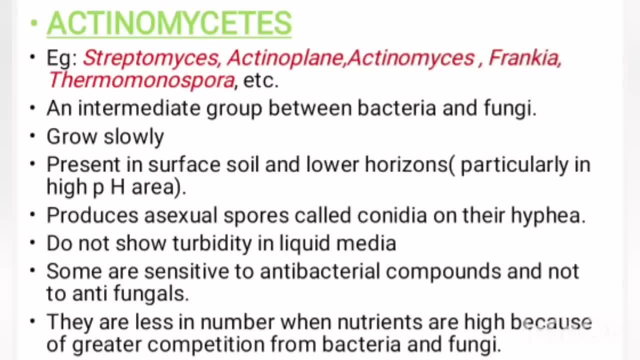 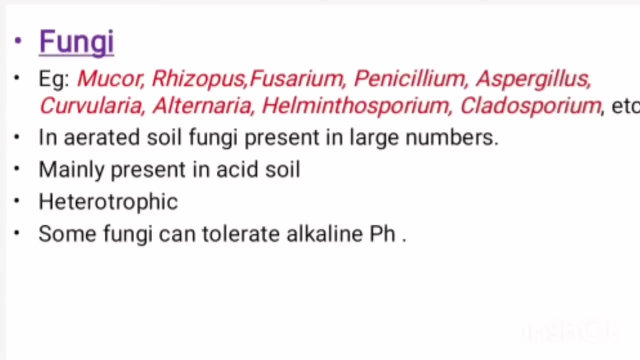 my sets are present in the surface soil and also in the lower horizon, particularly in environments of high PH and in in Japan. Third group of soil microorganism fungi. examples for the fungi are satas Wi. Hopefully I could have included the visible winners in my incorrect English translation. I hate uphill career. 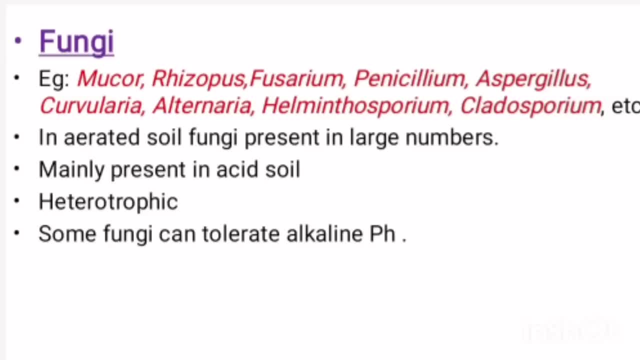 Fungi are mucor rhizopus fusarium alternaria, helminthosporium, cladosporium pensilium, aspergillus curvularia, etc. In well aerated soils, fungi are present in large numbers. 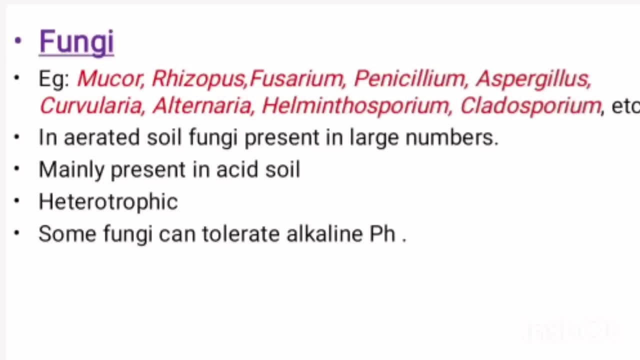 They are present in the form of mycelial beads, rhizomorphs or spores. Fungi are heterotrophic in nutrition. Some of the fungi can tolerate alkaline pH, ie pH beyond 9.. But fungi are not tolerant of alkaline pH. 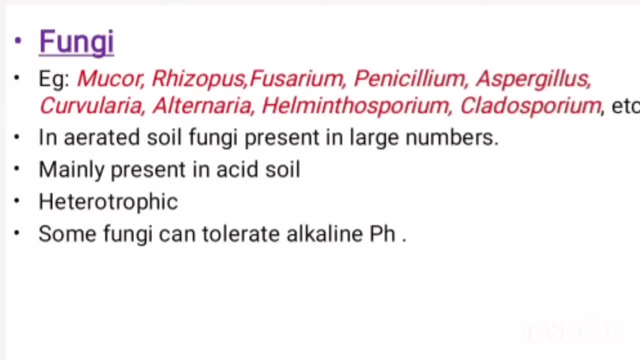 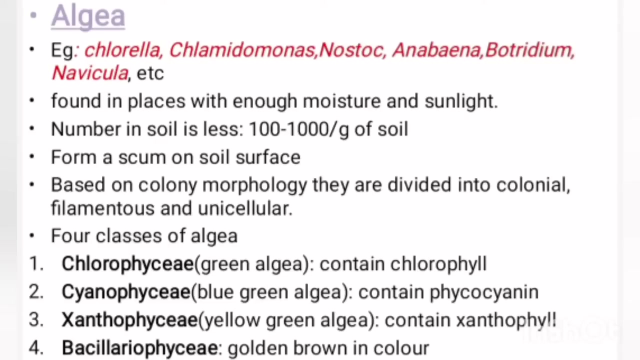 Fungi are mainly present in acid soil. Many factors influences the fungal population in the soil, which include pH, temperature, moisture, cultivation practice, inorganic nutrients, organic nutrients, depth, etc. Next one is soil algae. Algae are found in places. 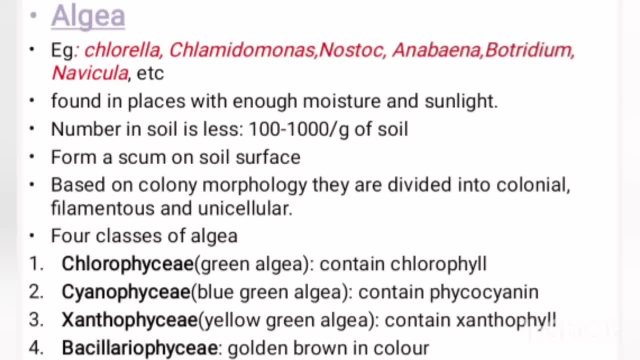 With enough moisture and sunlight. Some of the examples for the soil algae are Chlorella, Chlamydomonas, Nostoc, Anabena, Botrydium and Navicula. Their number in soil ranges from 100 to 10,000 per gram of the soil. 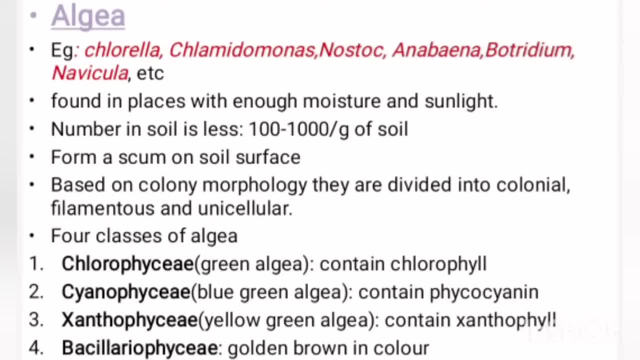 Their number in soil is less Compared to the bacteria and other organisms. Soil algae are divided into four classes, That are Chlorophyzae, Cyanophyzae, Cyanophyzae and Bacillariophyzae. 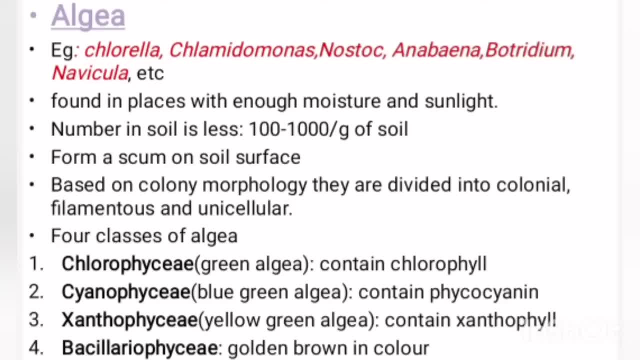 Ok, First one, Chlorophyzae. Chlorophyzae. It contains a green pigment called chlorophyll, So this algae is also called green algae. Example for the chlorophyzae are Chlorella and Chlamydomonas. 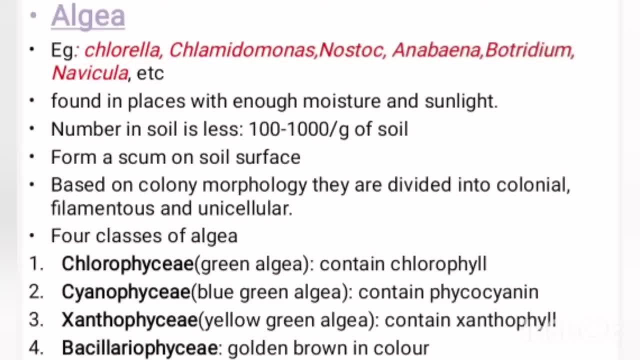 Second class, Cyanophyzae. It contains a blue pigment. Ok, That blue pigment is called Phycocyanin, So this Class is also called blue-green algae. Cyanophyzae is also called blue-green algae. 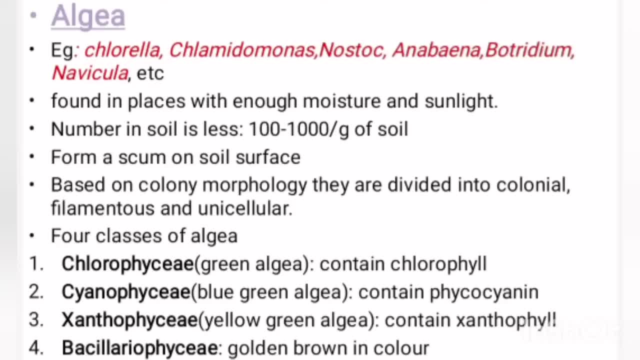 Because of that it contains a blue pigment called Phycocyanin. Example for the Cyanophyzae are Nostoc, Anabena, etc. Third class of soil algae is Sandophyzae. Third class of soil algae is Sandophyzae. 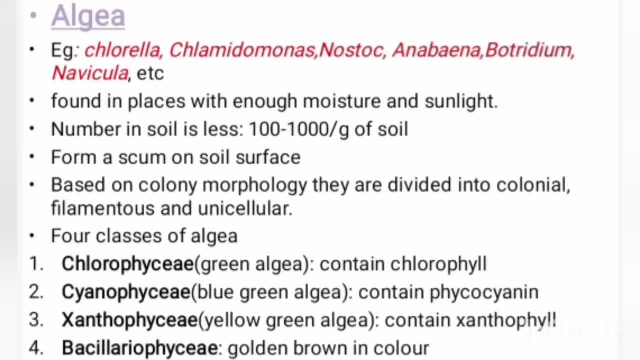 It contains a yellow-green pigment called xanthophyll, So it is also called yellow-green algae. Example: Botrydium. Then the last class of soil algae is Bacillariophyzae. They are golden-brown in color. 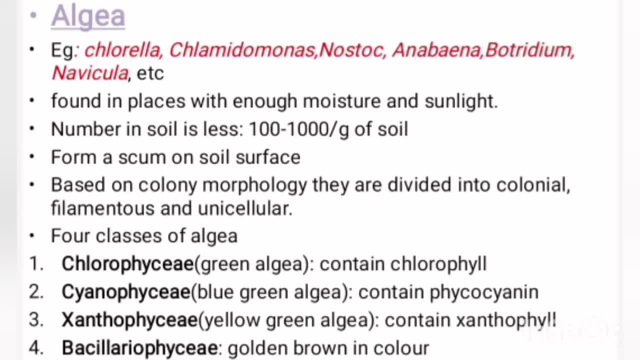 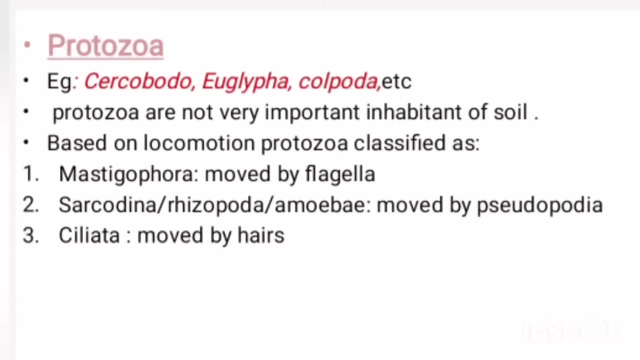 Example: Navicula. Based on the colony morphology, soil algae are classified into unicellular, filamentous and colonial. Fifth one: Protozoa. Example: Sercobodo, Euclipa, Colpoda, etc. Protozoa are not very important inhabitant of the soil. 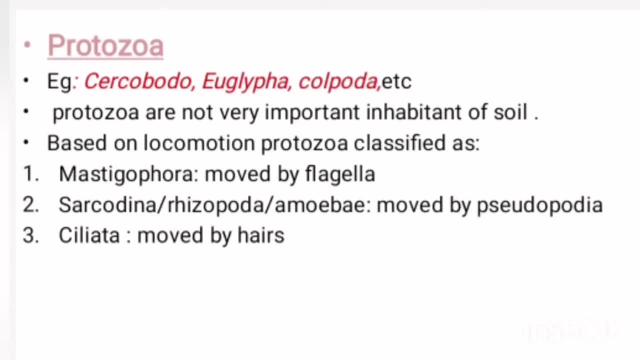 Soil. protozoa are classified on the basis of their means of locomotion, as Masticophora, Sarcodina and Celiata. Masticophora move by means of a long whip-like appendage, For example Sercobodo. 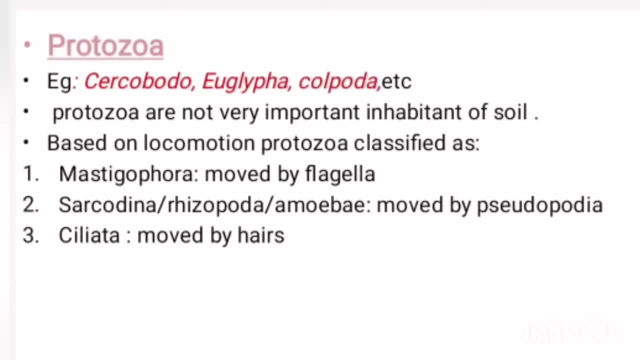 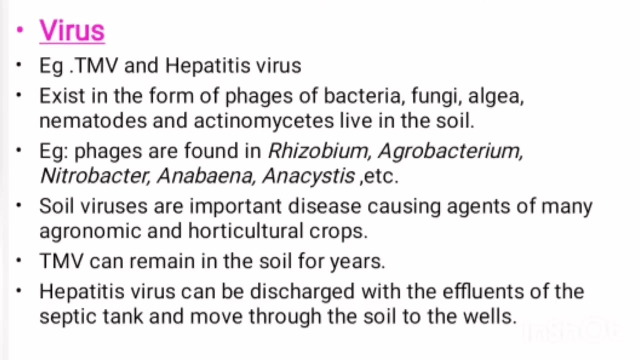 Second one: Sarcodina, or Rhizopoda or Amibe, Which is moved by Pseudopodia. Third one: Celiata. They contain hairs on their body which help them to move. Example: Colpoda powder. Last group of soil microorganism is virus. Soil virus exist in the form of: 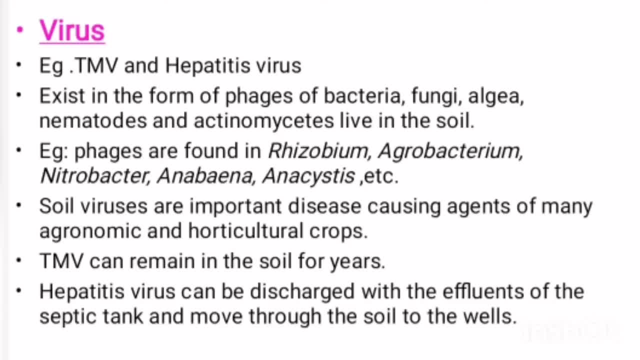 phages of bacteria, fungi, algae, actinomycetes, nematodes that live in the soil. Example phages found in rhizobium, agrobacterium, anasyst, etc. Soil viruses are disease-causing agents of many crops. 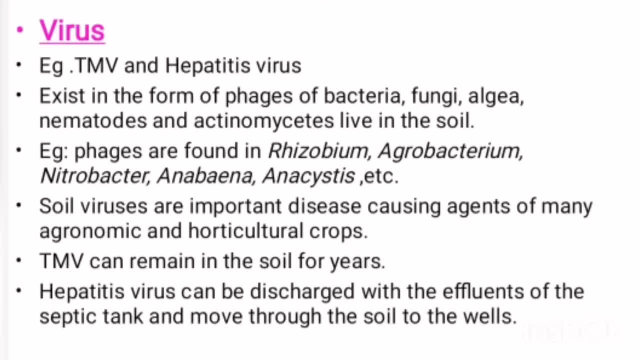 Some virus, like hepatitis virus, can be discharged with the effluents of the septic tank And then it moves through the soil surface then to the well or other underground water supplies. Another example for the virus is Tobacco mosaic virus, and this virus can remain in the soil for several years. 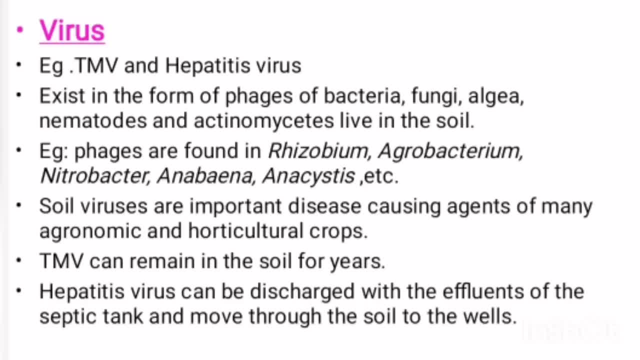 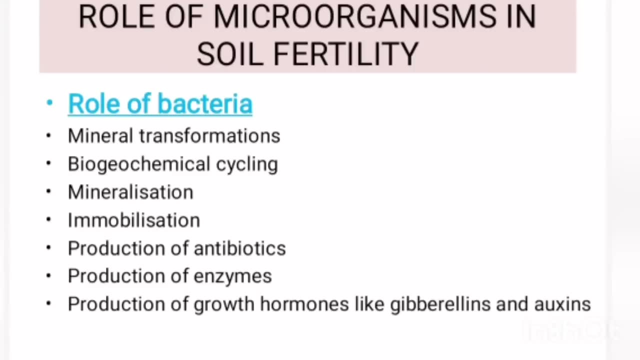 Ok, Most of the viruses remain active in the soil for long time. Role of microorganisms in soil fertility. Different types of organisms have different role in soil. First we can discuss the role of bacteria in soil fertility. All major mineral transformations or biogenesis. 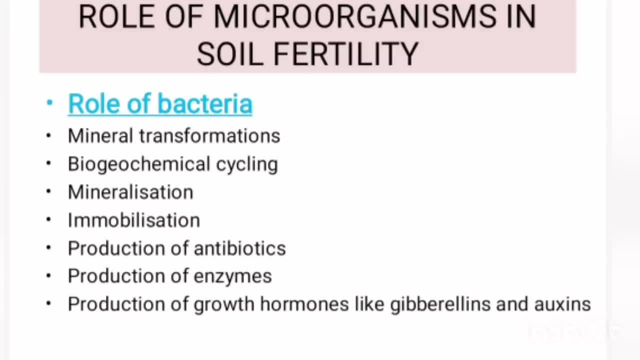 are present in soil. The geochemical cycling of nitrogen carbon, sulfur, phosphorus, iron, manganese and other elements are due to the activities of soil microflora: Mineralization, immobilization, production of antibiotics, production of enzymes, production of growth hormones like gibberellins and auxins. 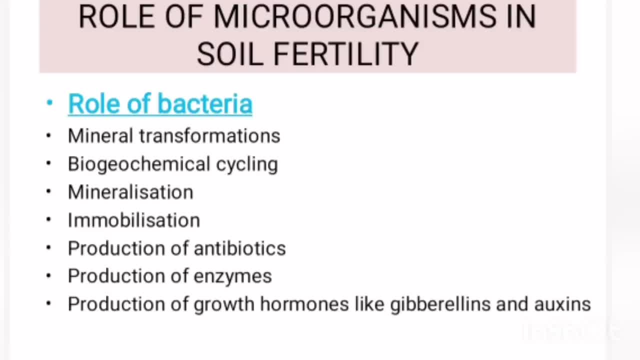 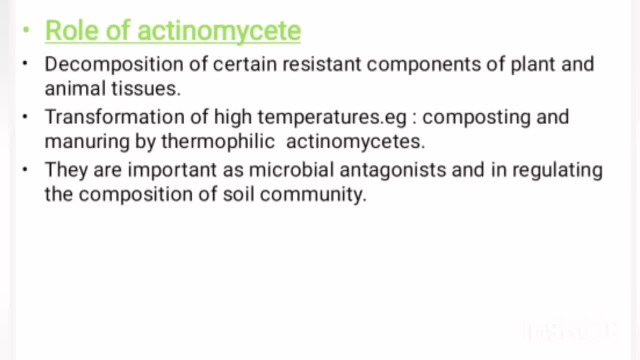 are carried out by the soil bacteria. Next, we can move to the role of actinomycete. Actinomycete participate in certain processes. First, the decomposition of certain resistant components of plant and animal tissues are carried out by actinomycete. Then the 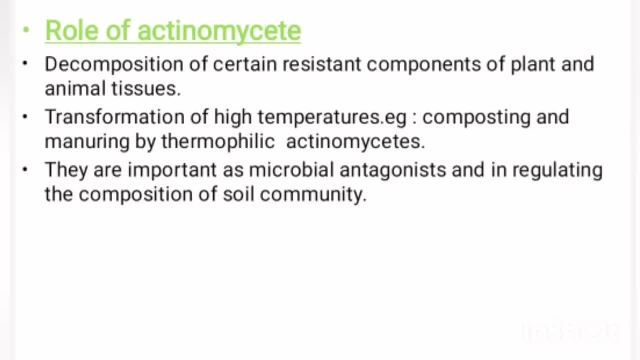 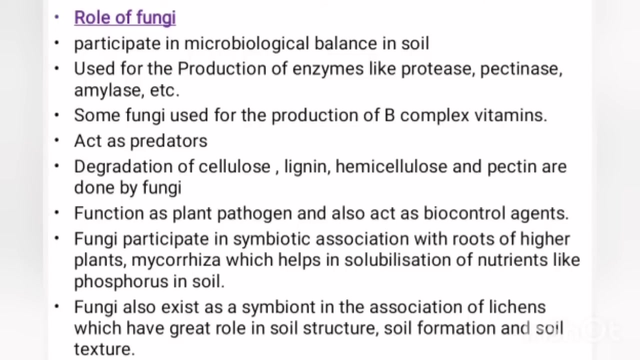 transformation at high temperature, example composting and manuring by thermophilic actinomycetes. They are important as microbial antagonist and in regulating the composition of bacteria Soil community. They also causes certain human infections like nocardiosis. Next is the role of fungi in soil fertility. Soil fungi play a major 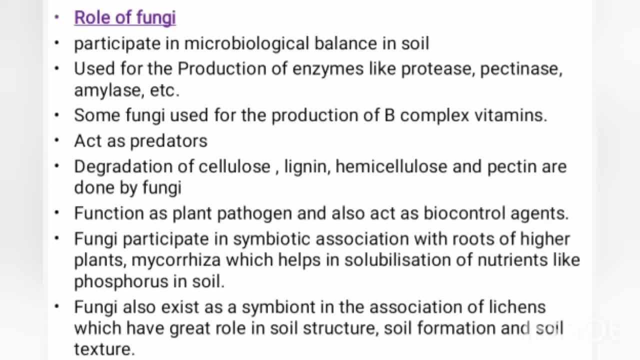 role in the manufacture of vitamin B complex and other vitamins, and also it is used for the production of industrial enzymes like amylase, protease, pectinase, etc. Fungi exist as symbiont in association of lichens, which have a great role in soil formation. soil. 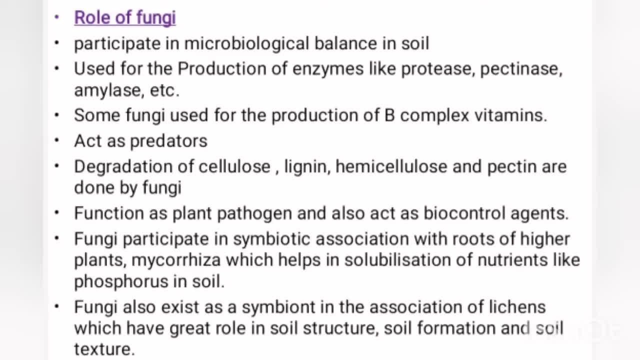 texture and soil structure, etc. Another important function of soil- sorry, another important function of fungi is the degradation of fabrics density, Degradation of complex soil. organic molecules like cellulose, lignin, hemicellulose and pectin are done by 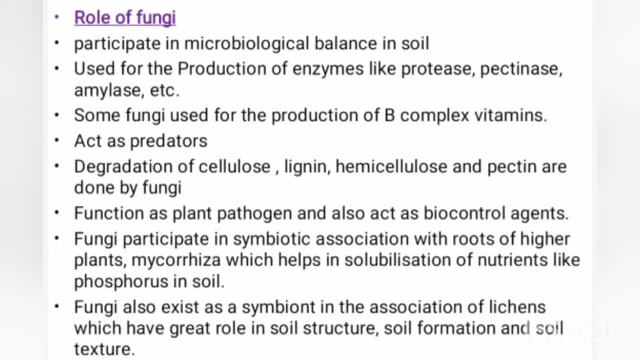 fungi. Fungi participate in symbiotic association with roots of higher plants, mycorrhiza, which help in solubilization of nutrients like phosphorus in soil. Unfortunately, it is notahuaca or strong- Mrs Valentine staples and other Mixedしか. 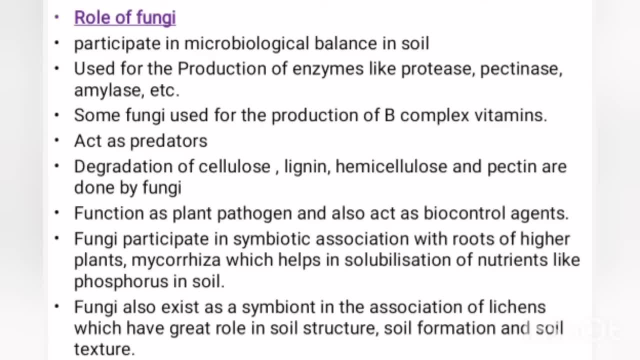 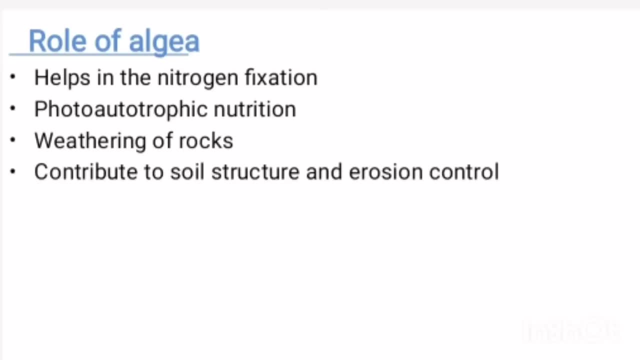 langella pollen costs. So so farachteifungae are the most-used, most popular B estrogliца in the acheiata fungi act as predators. another important function of the fungi is the microbiological balance in the soil. functions of soil algae. soil algae helps in nitrogen fixation, one of the